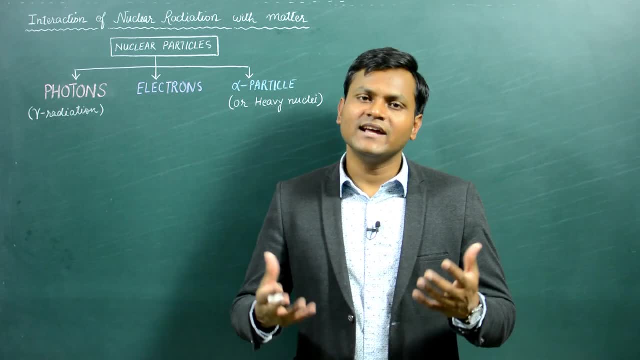 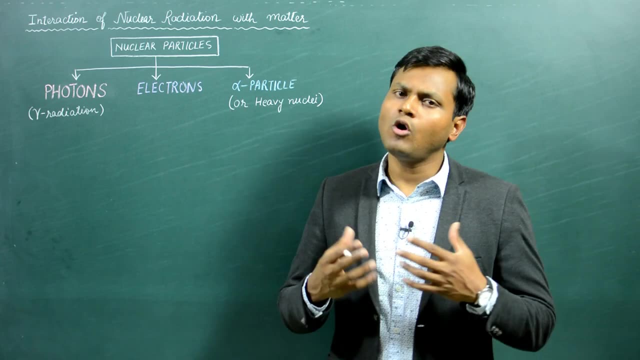 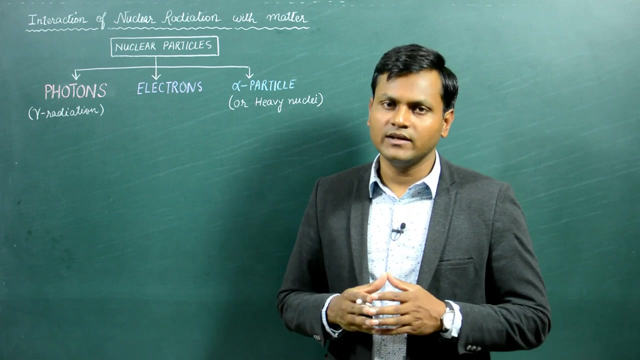 of tools or nuclear detectors which can detect different kinds of nuclear particles. So here I have classified the different kinds of nuclear particles that are emitted into three very common types. Now not all particles will fall in this particular category, but I'm just going to briefly discuss these three kinds of particles. So nuclear particles can. 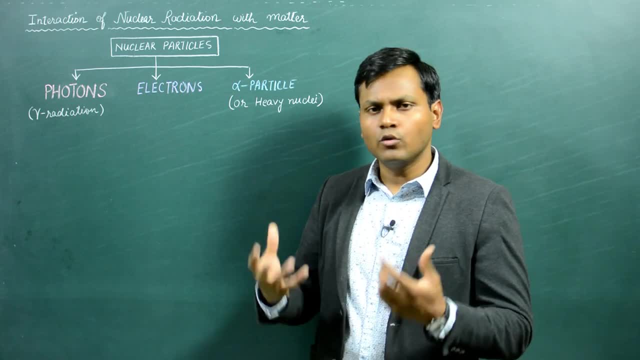 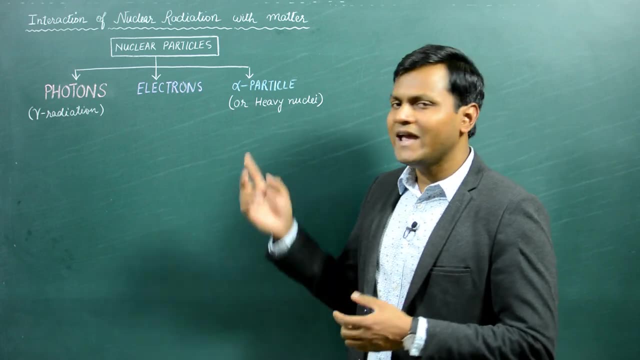 be categorized as either gamma photons or simply photons which are emitted in a nuclear reaction, or charged particles, One of them which could be electron or a positron, and the other is a particle or some other isotope or heavy charged nucleus Now, depending upon. 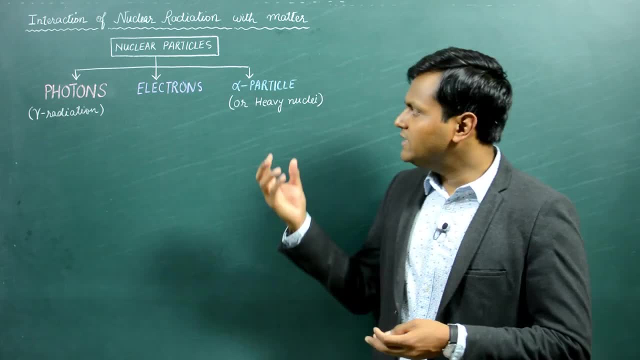 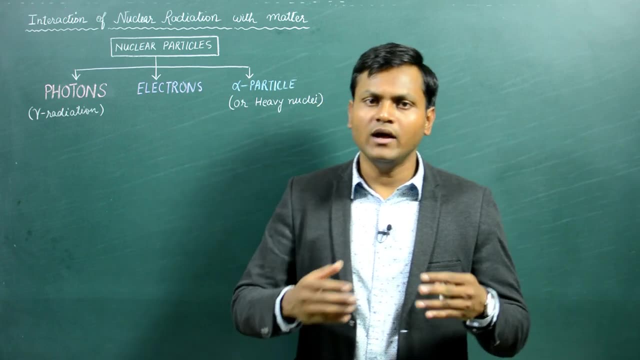 which particle is emitted in a nuclear reaction, it can induce different kinds of phenomena when it enters a material medium. So let's discuss those kinds of phenomena separately for each of these particles. So let's first talk about the case of photons. So whenever 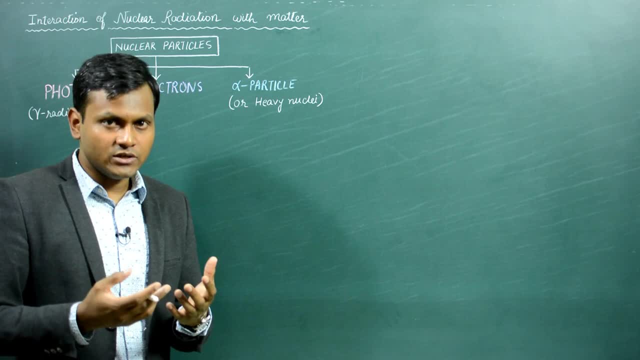 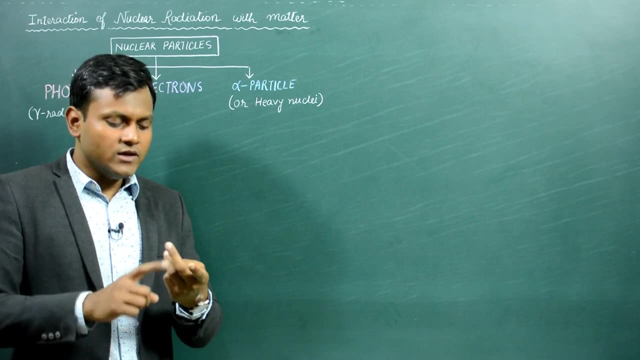 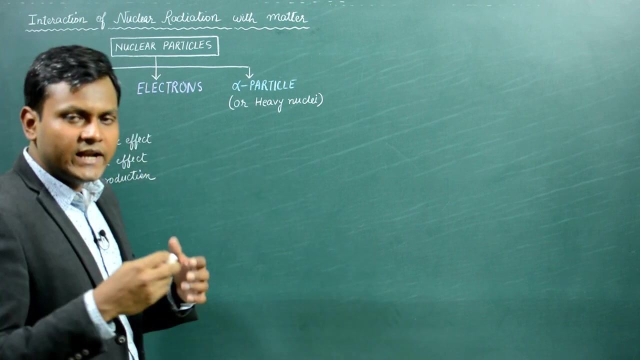 gamma radiation is emitted in some kind of a nuclear reaction. that kind of a gamma radiation can lead to different kinds of phenomena in a material medium. Very common phenomena are the photoelectric effect, the Compton effect and pair production. So whenever gamma photons enter a material medium they can induce any one of these three. 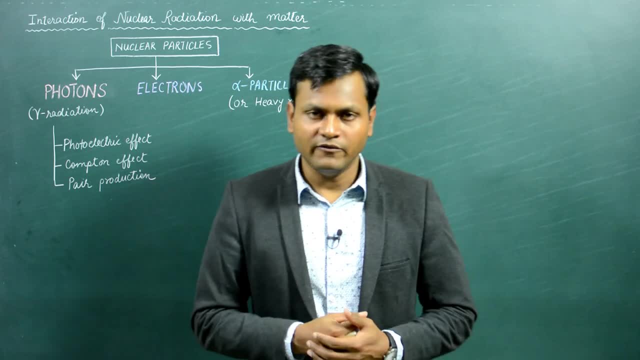 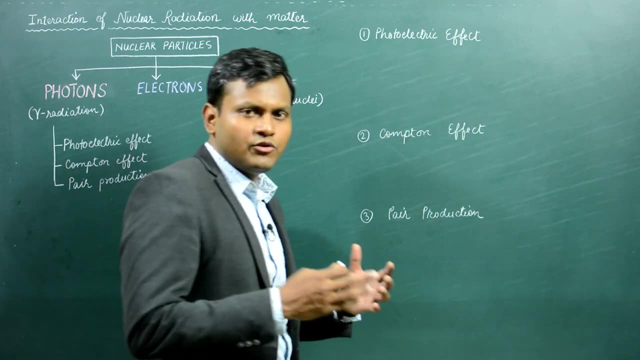 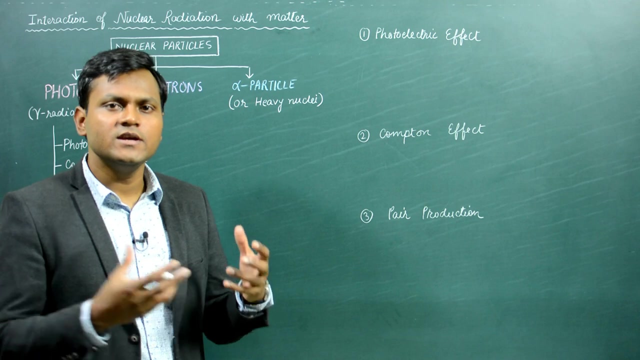 phenomena, depending upon what is the energy of the gamma photon. So let's discuss these three individually. Now. all of these three effects involve incident radiation or an incident photon. However, the effects of the incident photon are different. So let's talk about the first case: photoelectric effect. What is photoelectric? 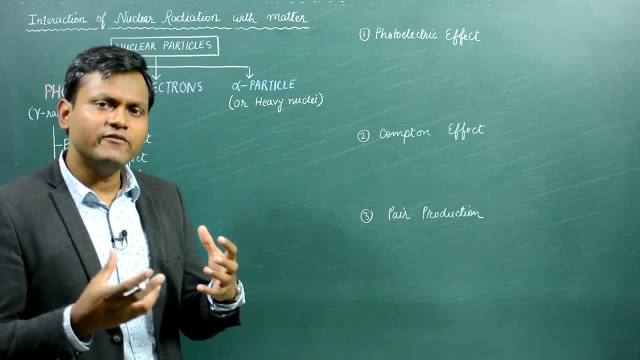 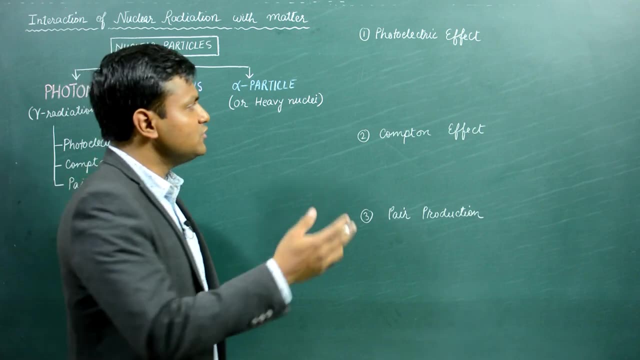 effect. The simple definition of a photoelectric effect is that whenever some sort of a radiation is incident onto a surface and it leads to the ejection of electrons, then that kind of an effect is known as photoelectric effect. So in the case of a photoelectric effect, 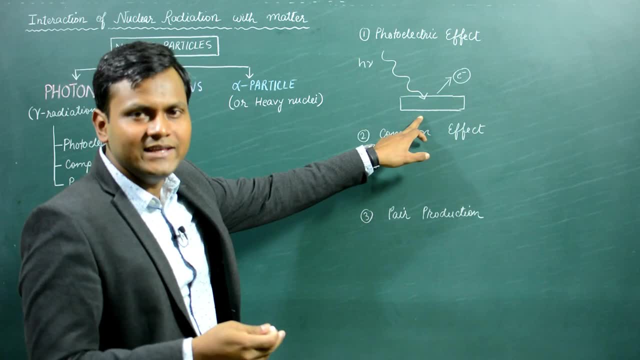 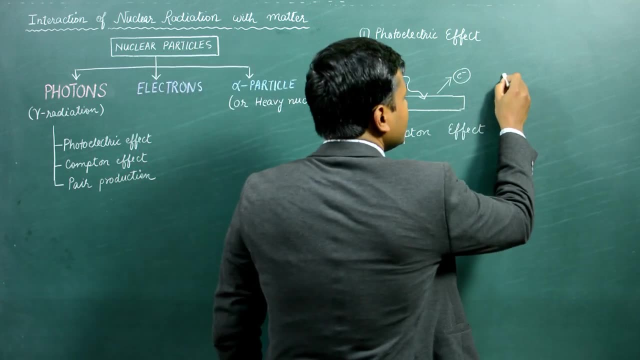 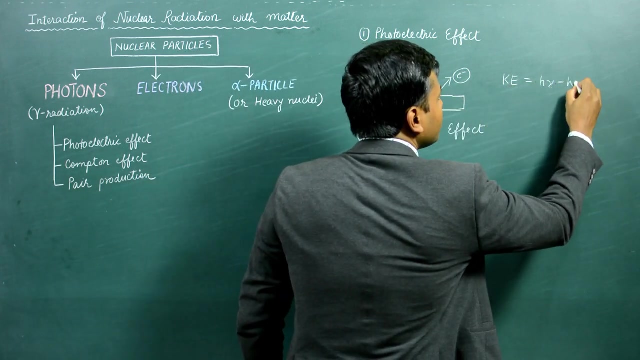 when some sort of a nuclear gamma radiation enters a material medium, then it leads to the emission of free electrons. The kinetic energy of the electron is given by. the kinetic energy is simply the energy of the gamma photon, which is h, nu minus the work function of the material. This is basically. 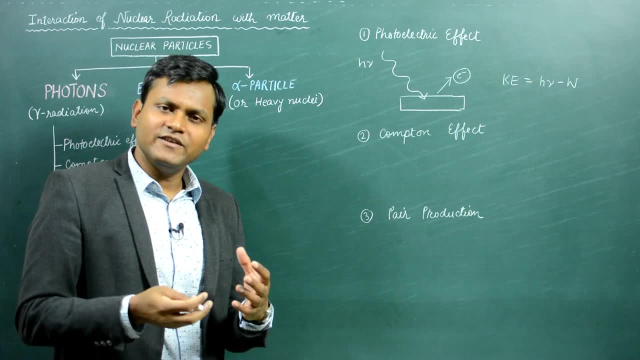 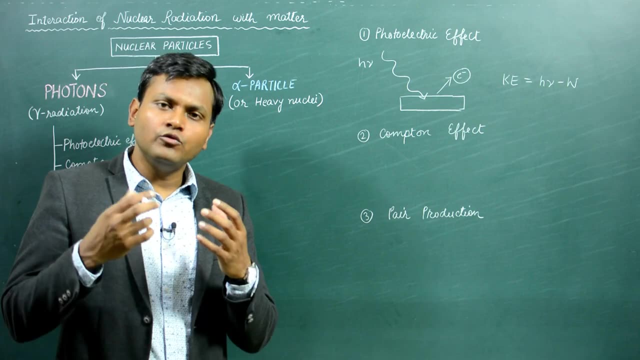 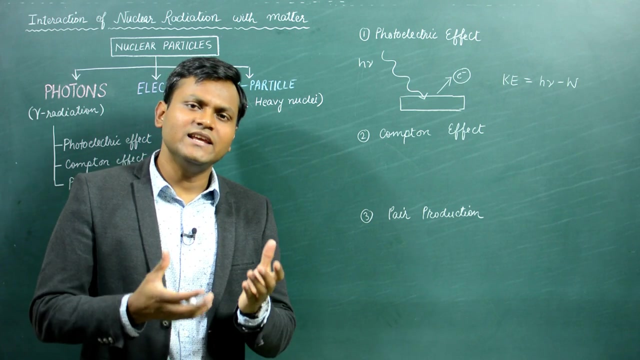 known as the Einstein's photoelectric equation. Now, understanding photoelectric effect is quite simple, because electrons are usually stuck to the individual atoms inside a given material. Now, to free these electrons you need certain amount of energy. Whenever an incident- nuclear radiation falls onto a material medium, it basically interacts with the electrons'. 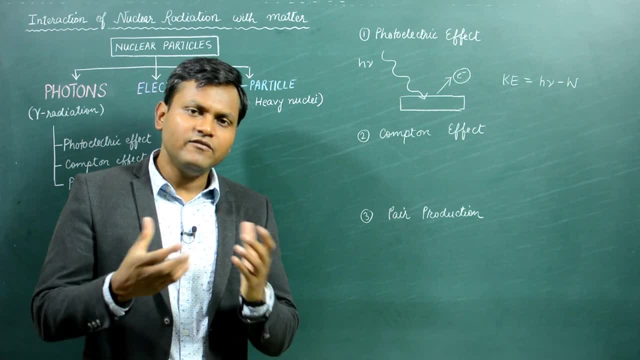 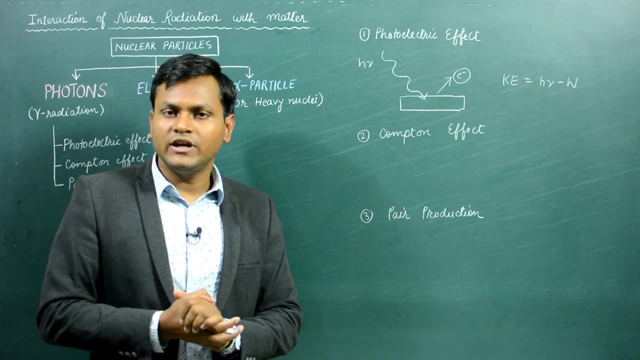 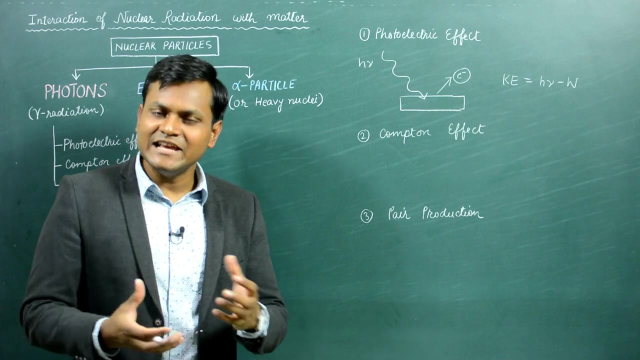 electrons which are stuck in the atomic structure of an atom. If the energy of the incident radiation is sufficient, then the electron can absorb that energy and become free from the potential of the atom itself. The excess amount of energy usually gets converted to kinetic energy of the electron, Since the ionization energy of the electrons is not. 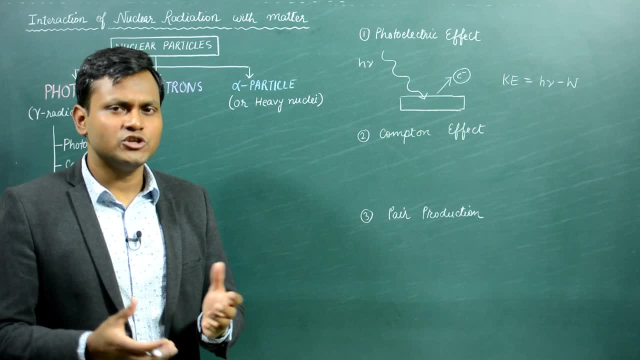 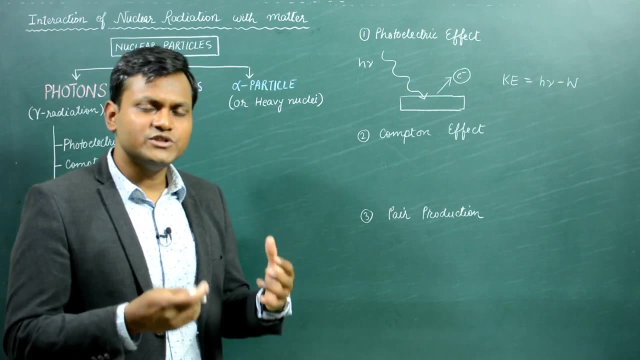 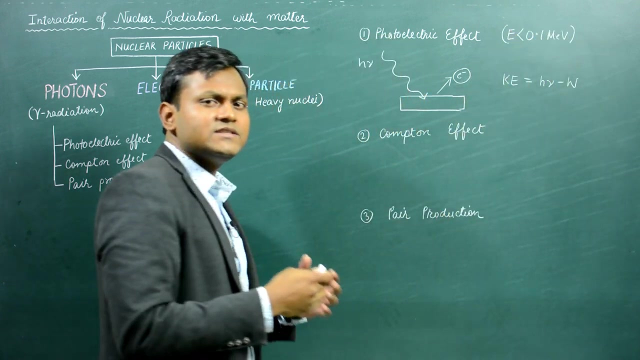 very high to induce photoelectric effect. we do not need an extremely high energetic photon. Photoelectric effect is usually seen for low energetic photons or photons which have energies less than 0.1 mega electron volt. So photoelectric effect is usually seen. 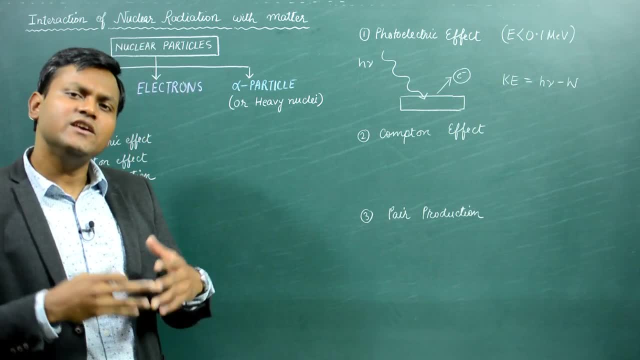 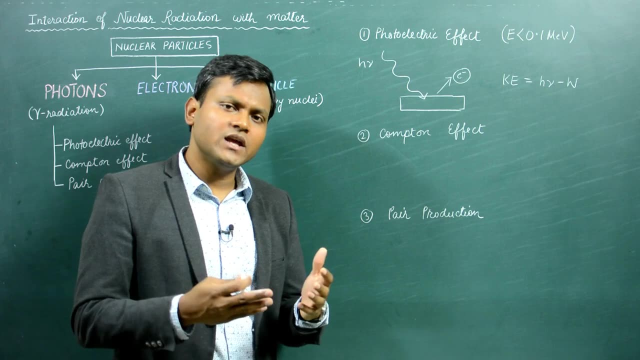 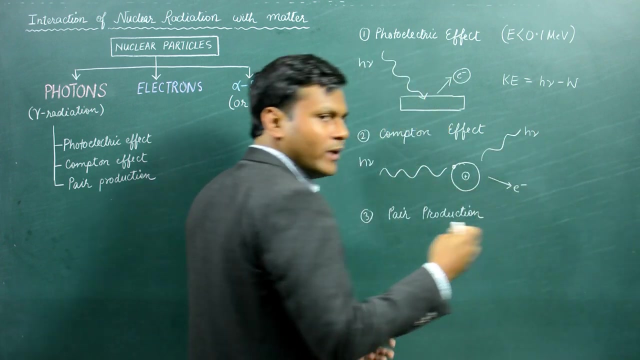 for gamma photons, which have extremely less energy, and the effect of this is just freeing up of electrons or ionizing the material. Next phenomena is that of the Compton effect. The Compton effect occurs for usually a little bit higher energetic photons. So whenever 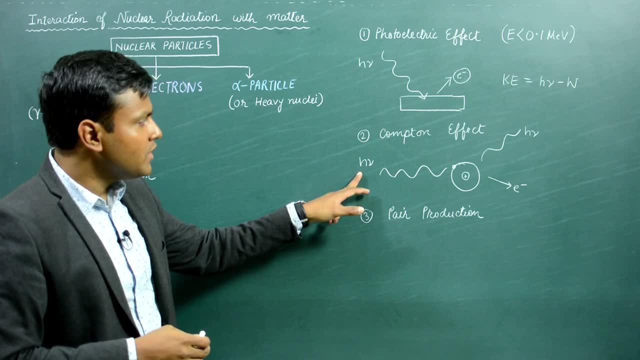 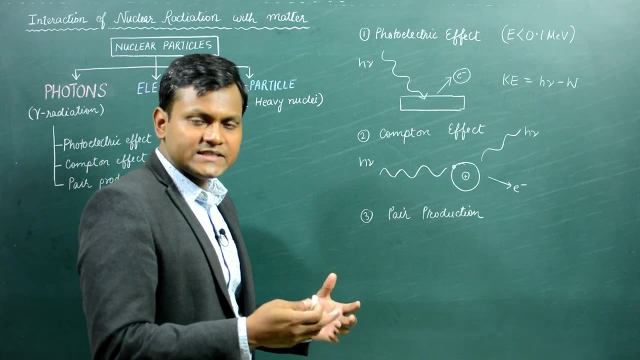 some kind of a high energetic photon having energy h nu interacts with the electron, then it interacts with some kind of an electron which might be stuck in an atom or might be a free electron. In that case, first of all, because the photon has extremely high 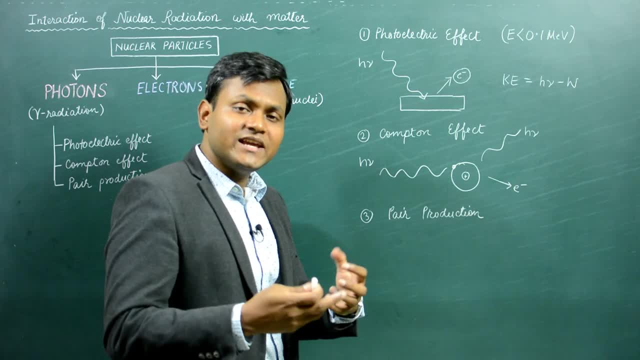 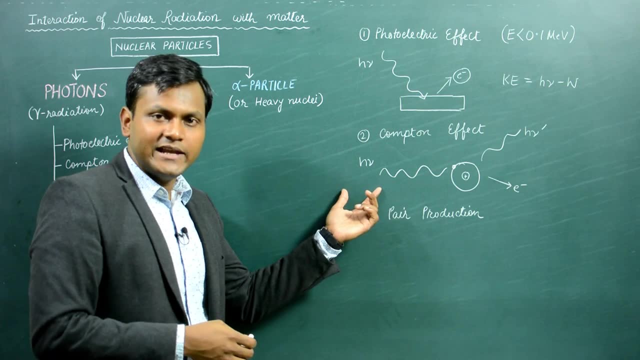 energy, it will free up the electron and it will elastically scatter from the electron. So you will also have scattered radiation having certain frequency which is less than the incident radiation. Now this phenomena is known as the Compton effect and the equation. 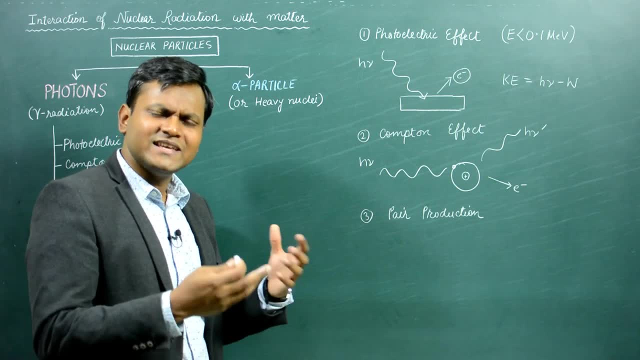 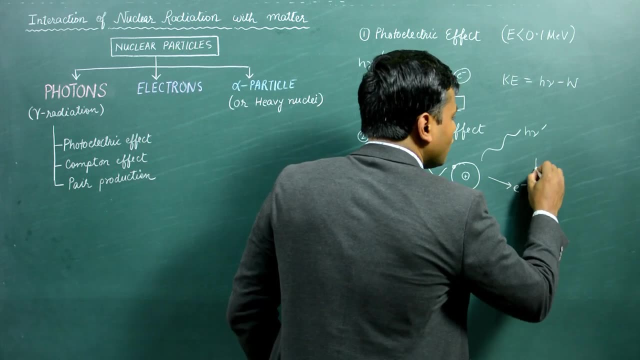 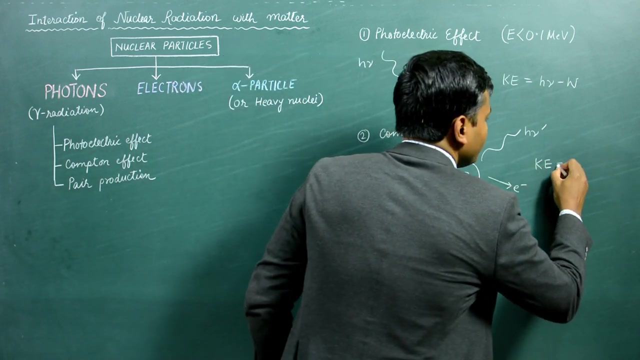 associated with the Compton effect is known as Compton's equation, which basically gives us the change in the frequency of the incident radiation. In this case, the kinetic energy of the electron simply comes from the change in the energy of the incident radiation and the scattered radiation. This equation is true for free. 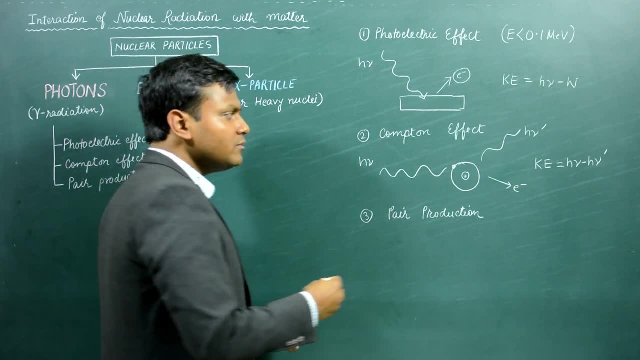 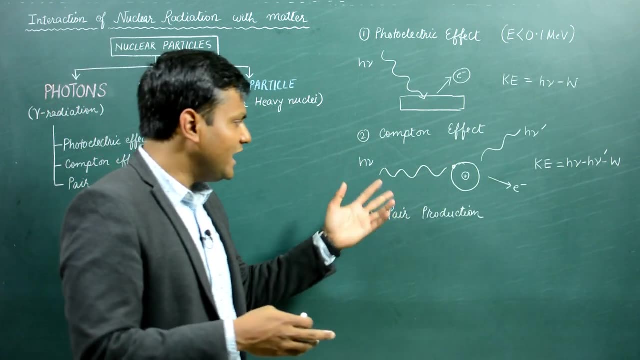 electrons. If the electron was originally stuck to some kind of an atom, then you will have to subtract the work function or the ionization energy of the electron. So the high energetic photon not only ionizes the material medium but also gets scattered from. 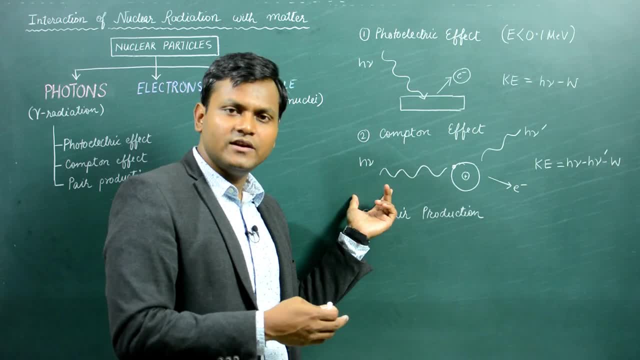 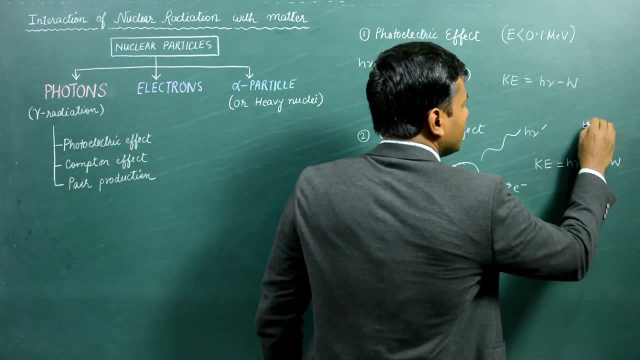 the material medium with some sort of a frequency less than the incident radiation. So the high energetic photon not only ionizes the material medium but also gets scattered from the material medium with some sort of a frequency less than the incident frequency. So this kind of a phenomena is usually dominant for energy of photon having range from greater. 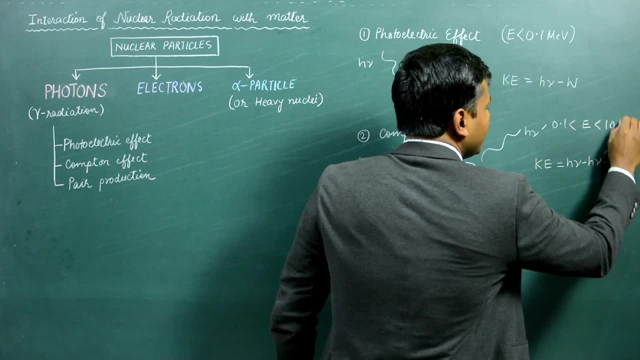 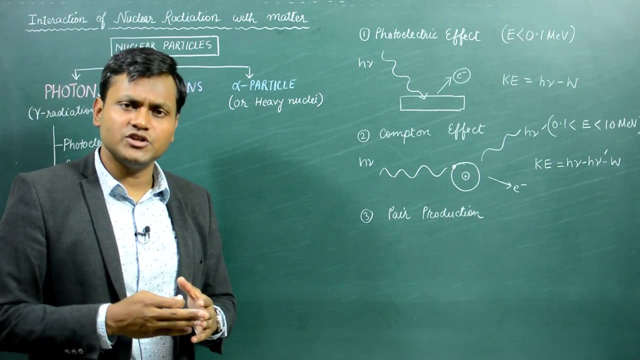 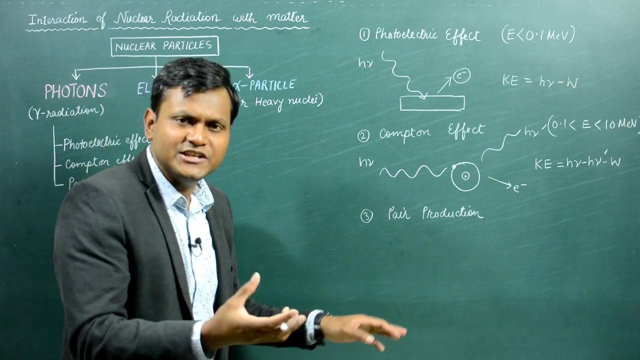 than 0.1 mega electron volt up to 10 mega electron volts. The next phenomena for photons having even higher energy, for extremely high energetic photons, is known as pair production, Now pair production. to understand pair production you need to understand pair annihilation. So pair annihilation is extremely simple. 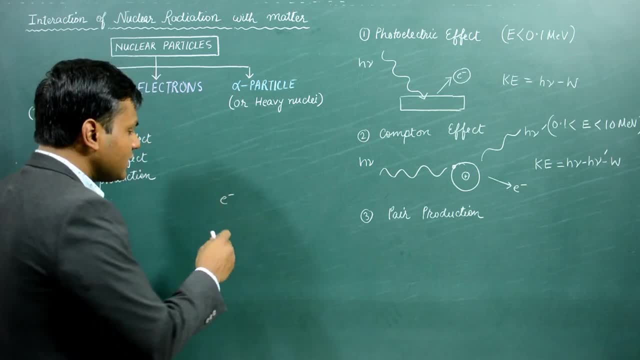 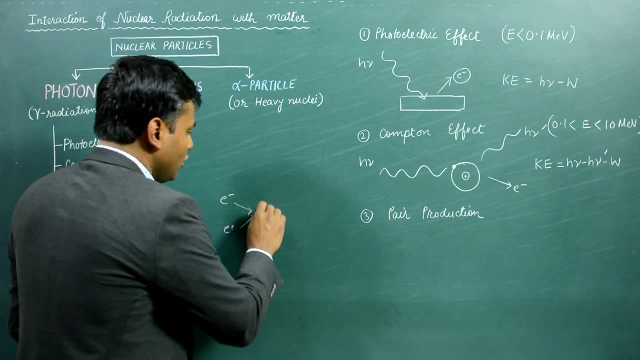 A matter particle- let's suppose an electron and its antimatter version- let's suppose a positron- comes together, then they lead to the creation of pure energy. Now the reverse to this kind of a process is also possible, The reverse to this kind of a process where 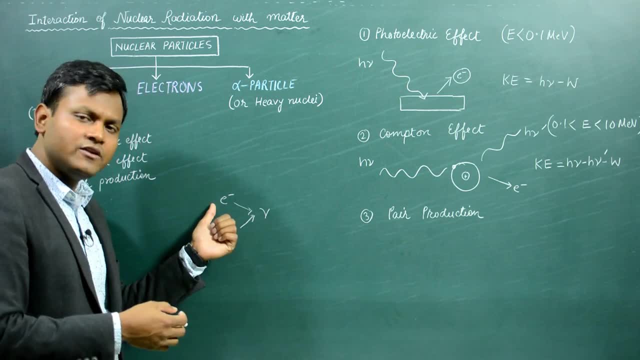 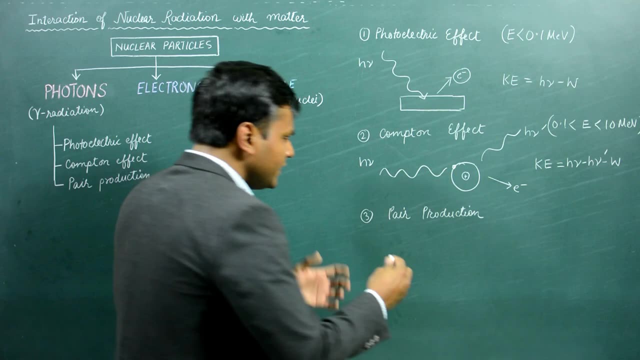 pure energy can get transformed into a matter version of an electron, and an antimatter version of an electron is known as pair production. So whenever some extremely high energetic gamma photon comes close to some kind of a produced energy, a pair production is called pair production. So whenever some extremely high energetic gamma photon comes close to 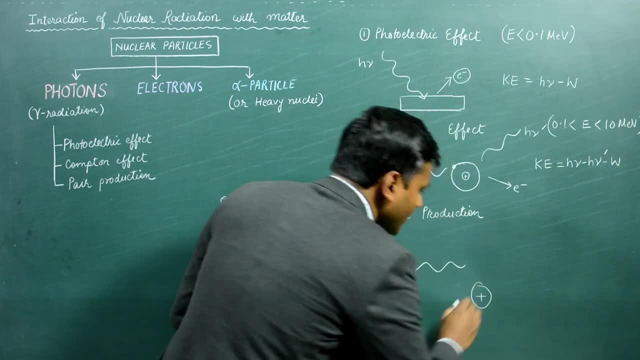 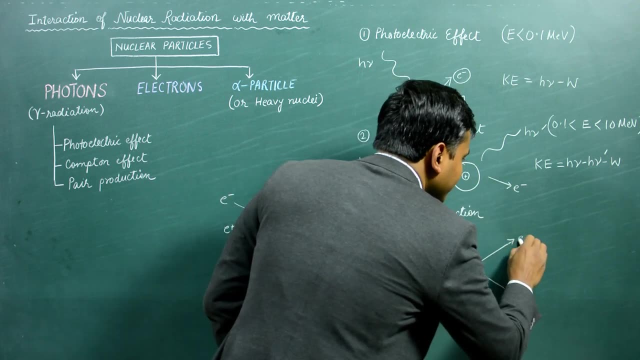 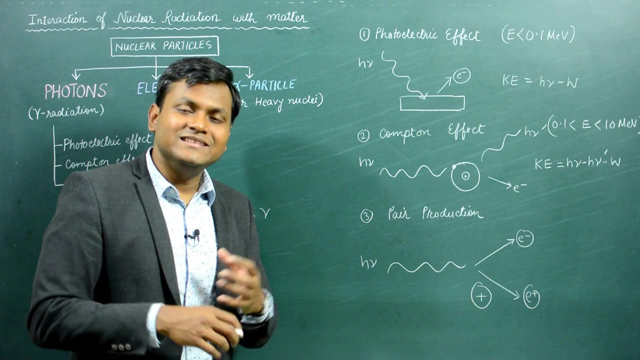 some kind of an external nucleus, then in the potential field of that particular nucleus, the energy of the gamma photon can lead to the creation of an electron as well as a positron. Now, since radiation energy is creating matter, the energy of the radiation must be greater than. 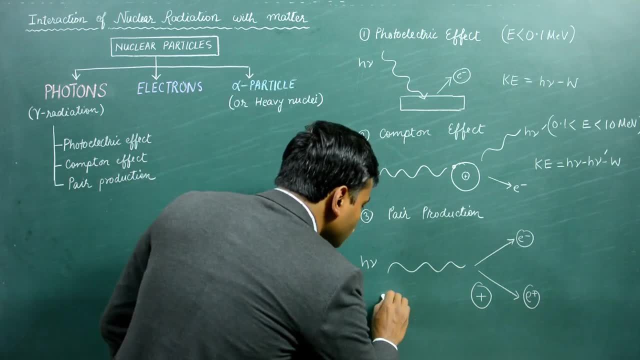 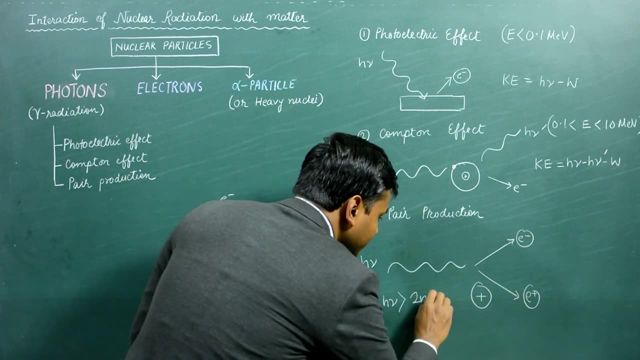 the rest mass energy of both of these particles. So h nu, the energy of the photon must be greater than the rest mass energy of both the electron as well as the positron. Therefore this kind of a process is not possible for low energetic particles. 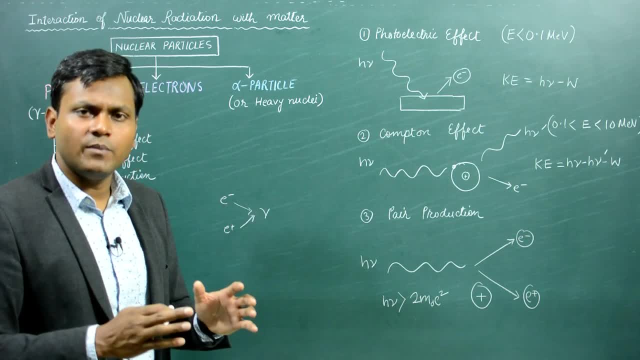 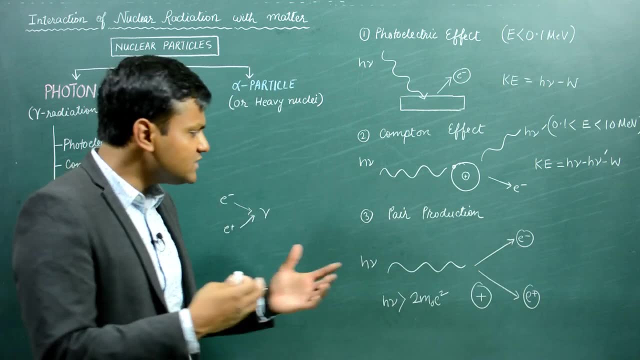 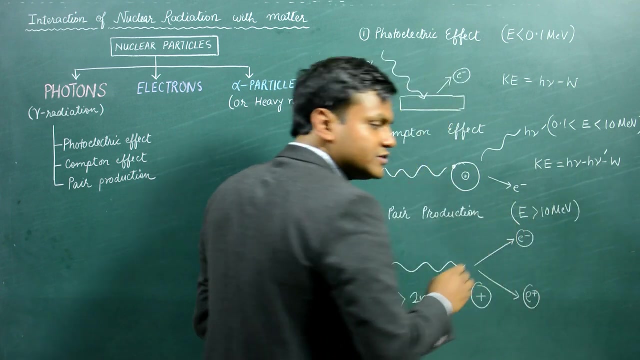 This kind of a process only happens for extremely high energetic particles, which has sufficient amount of energy to create this kind of electron and positron pair in the first place. So this kind of a process is usually dominant for energies greater than 10 megaelectron volts. 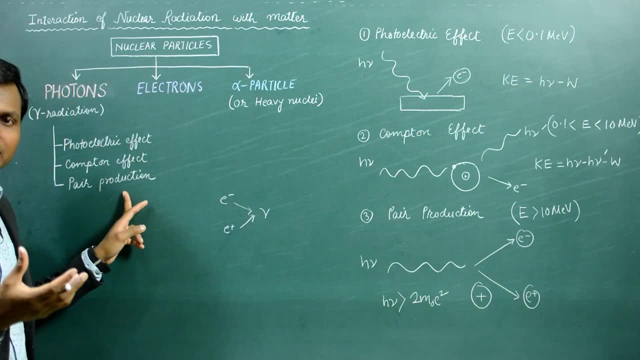 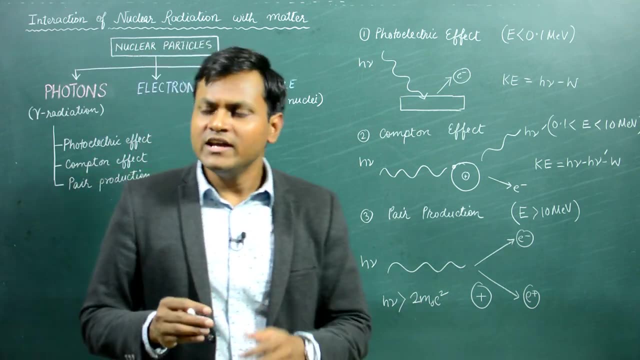 So, as you can see, for the same kind of a photon as an electron ion is海 window, there is a Curren call pass into the counter particle emitted during some kind of a nuclear reaction. we can see three different kinds of phenomena, based upon whether or not the energies of the 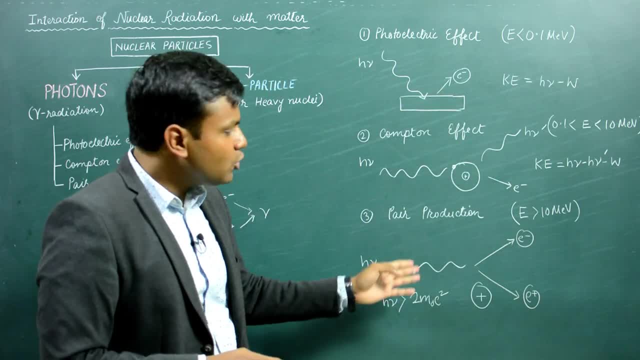 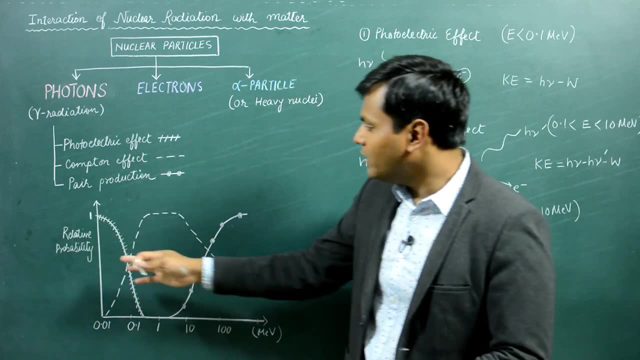 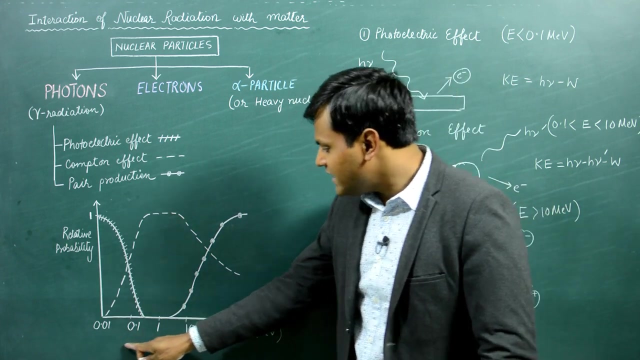 photon particle is low, medium range or extremely high. we can demonstrate this using a particular graph. so here I have drawn a graph which shows the relative probability of a particular phenomena happening whenever some photon interacts with a material medium. so, as you can see here, as the energy of the photon keeps, 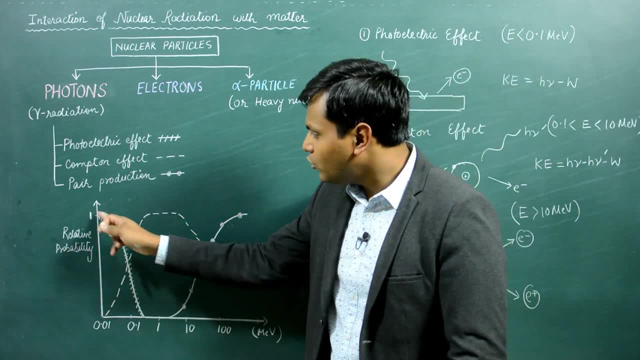 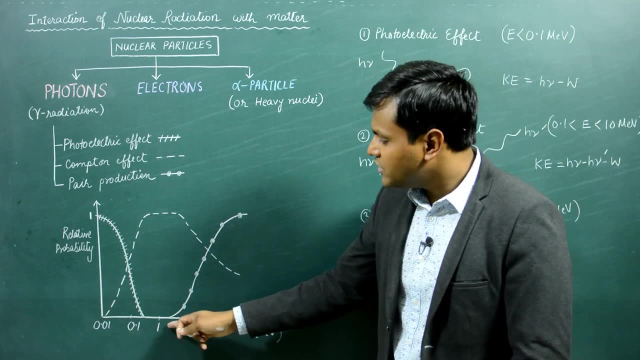 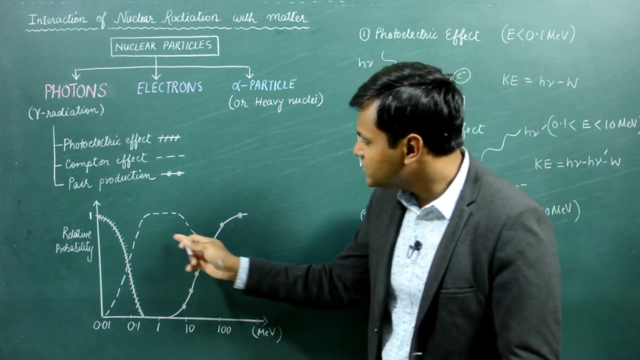 on increasing. initially for low energetic photons, the photoelectric effect is dominant. slowly the Compton effect starts dominating and at the end you have, for extremely high energetic photons, the pair production starts dominating. so, as you can see here, these three different main phenomena which are represented by these three different graphs, show the different kind of 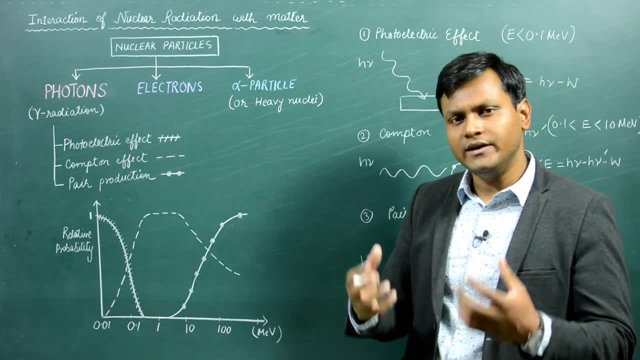 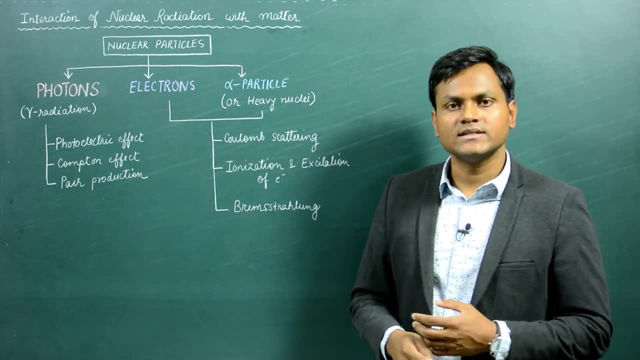 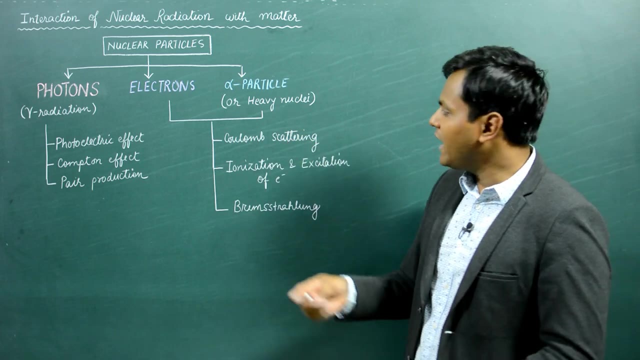 phenomena that arises whenever photons of different energies enter a material medium. now, next, we come to the case of charged particles like electrons and alpha particles. now, charged particles like electrons and alpha particles usually exhibit any number of phenomena. out of these three, we have the Coulomb scattering. we have 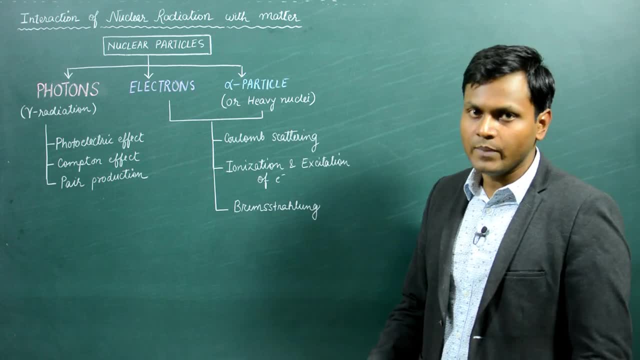 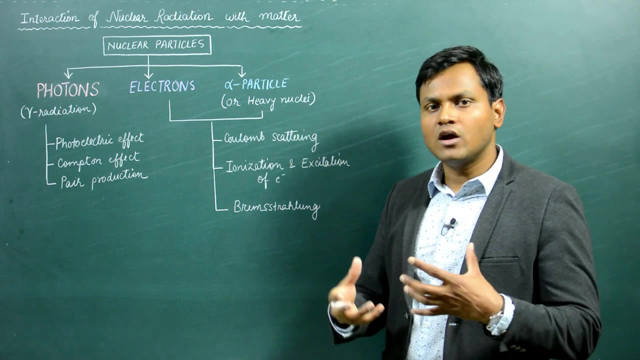 ionization and excitation of electrons and the Bremsstrahlung effect. so usually the electrons exhibit either ionization or the Bremsstrahlung effect, and the alpha particles or some kind of a charged heavy nuclei exhibit Coulomb scattering and ionization. now let's discuss these phenomena one by one. what 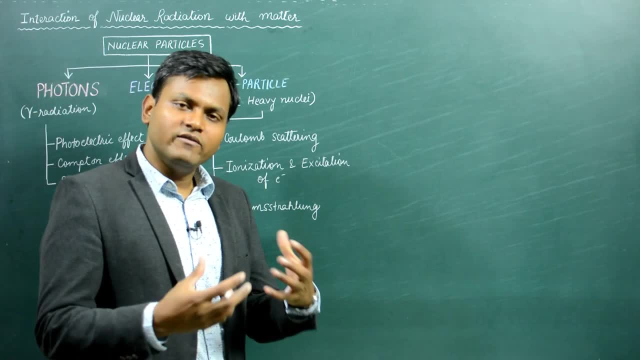 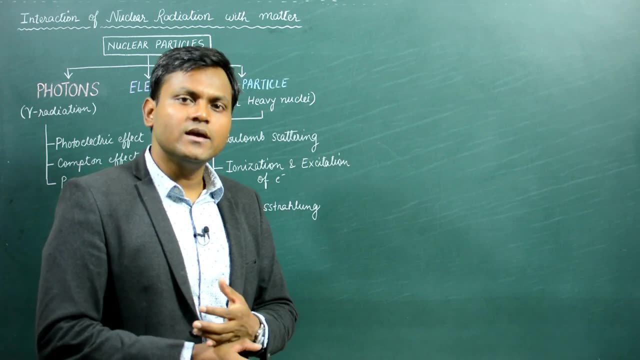 is Coulomb scattering? Coulomb scattering is a very simple phenomena. whenever a positively charged nuclear particle is charged with a positive charge, it will. particle comes into the coalympic field of a given target nucleus, then it usually experiences repulsion and it changes its trajectory. So whenever some 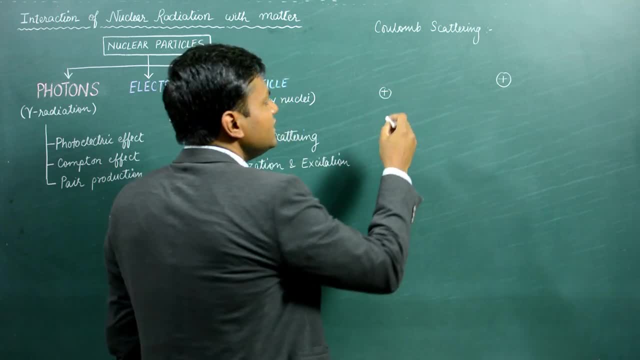 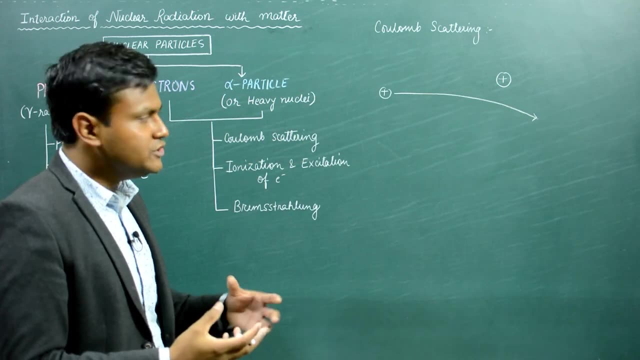 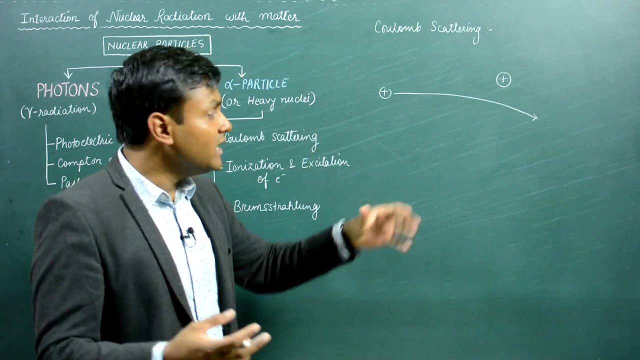 kind of an incident charge particle comes in the vicinity of a target nucleus, then it usually changes its trajectory if it does not have sufficient amount of energy to penetrate through the coalympic repulsive barrier of the target nucleus. If the incident particle was extremely high energetic, it would 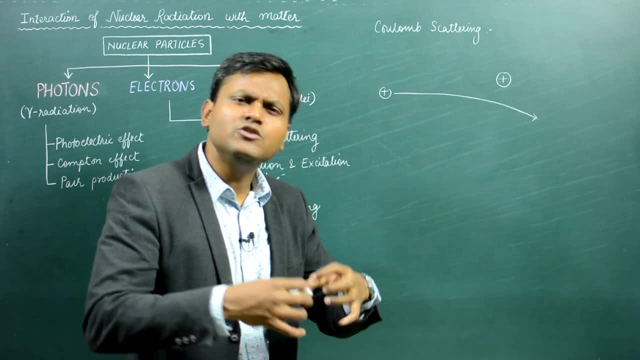 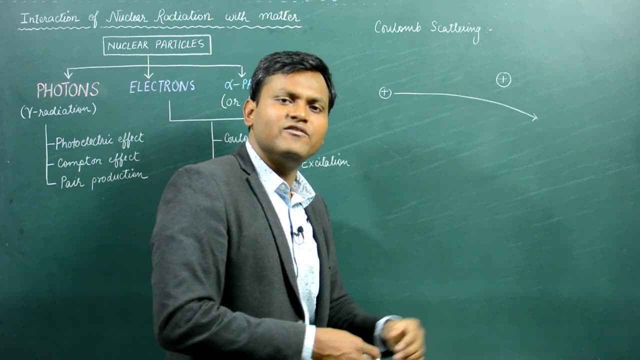 penetrate the coalympic barrier and interact with the nucleus and lead to some sort of a nuclear reaction. but if the energy is not sufficient enough then it will easily get repelled and just get deflected in different directions. The second and the most common kinds of phenomena that is seen whenever either. 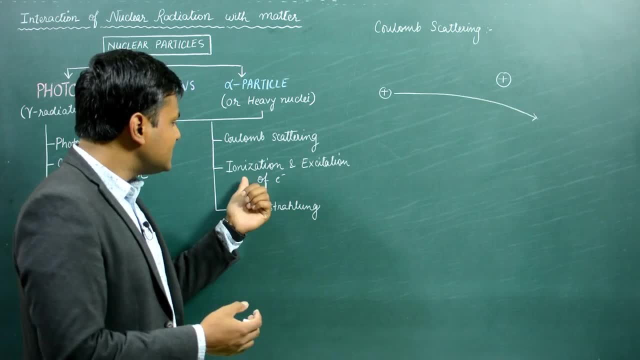 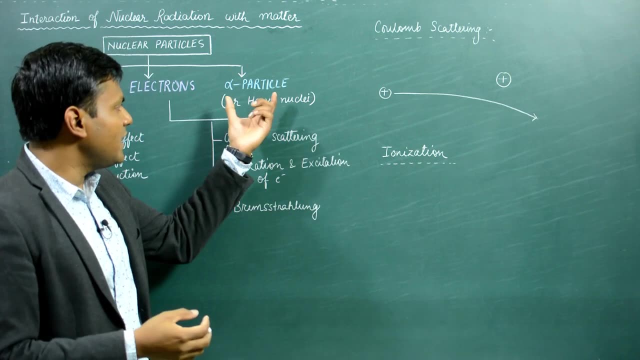 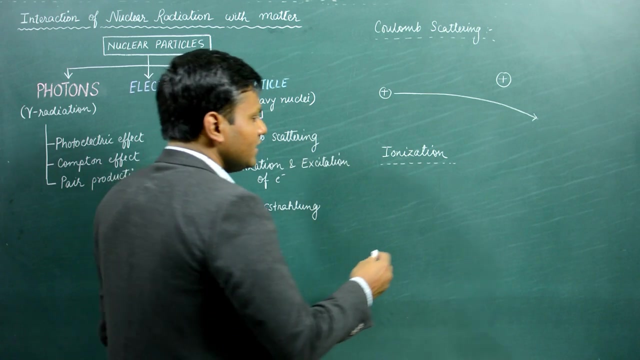 an electron or an alpha particle enters a material medium is that of ionization. So ionization, or excitation, is simply the phenomena of some external nuclear particle interacting with the atoms of the nuclear system. So ionization is a form of these parameters. term toойд dot Entertainment, One of the main. 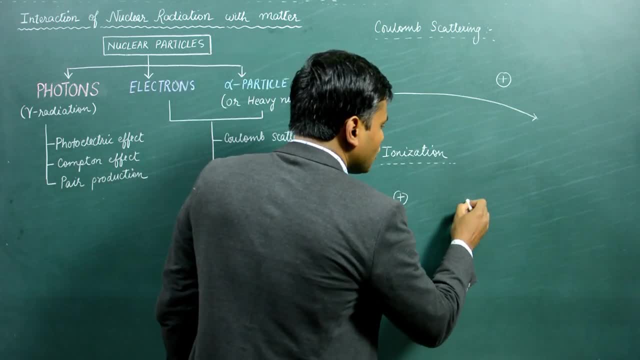 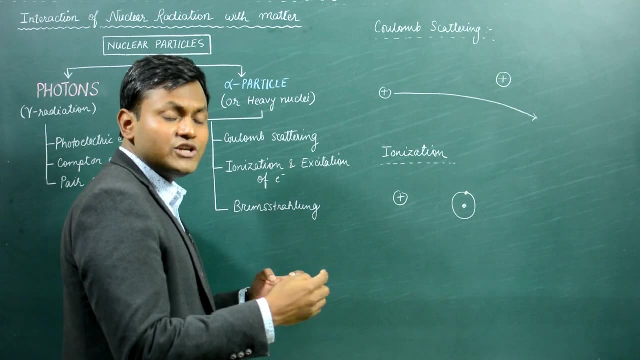 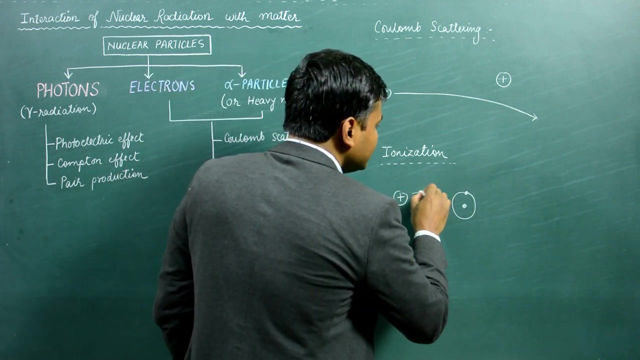 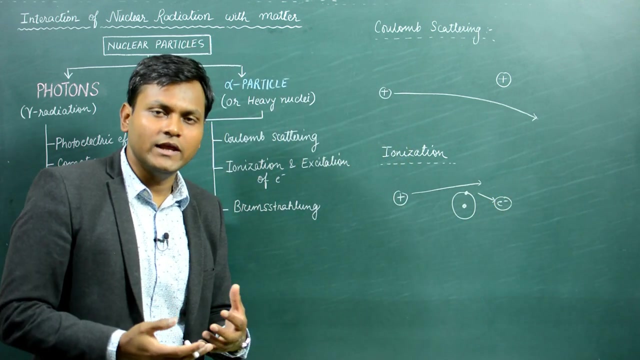 reasons why ionization is important is by rise of alcohol, Event behavior, attract, collect if PROFESSOR, and that would lead to the creation of free electrons and positively charge target nuclei. Now, usually alpha particles which are emitted in nuclear reactions are a very high energetic. They usually have energies of the order of 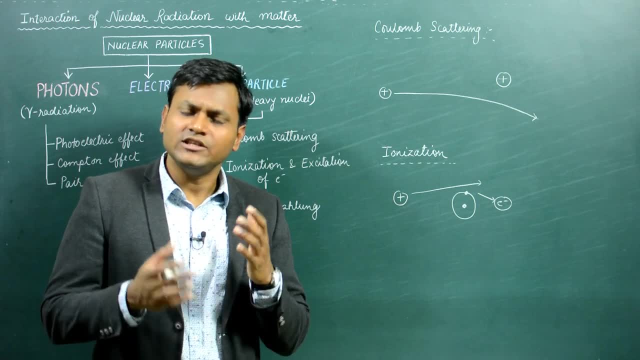 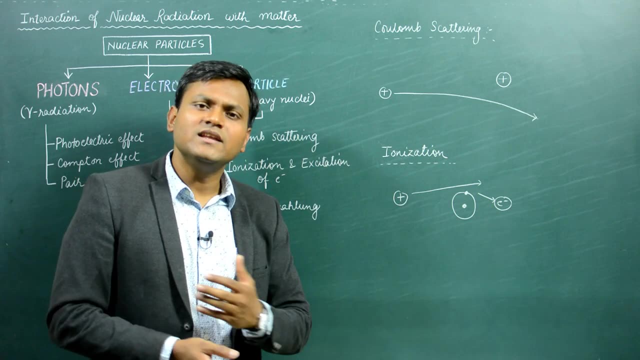 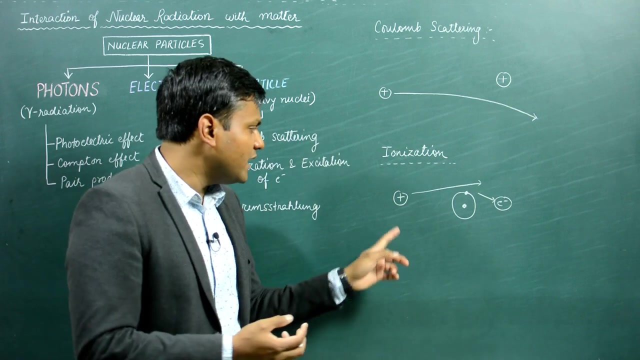 4 to 10 mega electron volt. That is huge amount of energy compared to the ionization of an energy of an electron stuck in an atom. So electrons usually need a couple of electron volts to become free from the atomic nucleus. So whenever an alpha particle is incident onto some kind of a material medium, then 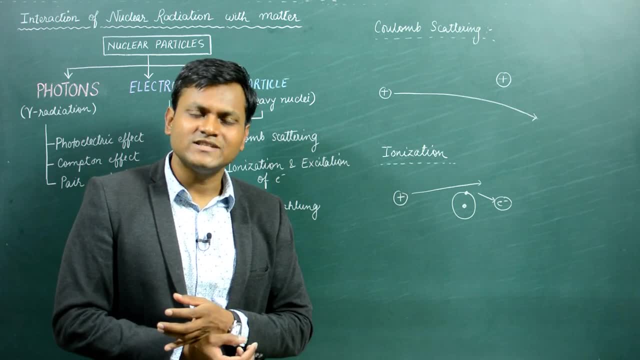 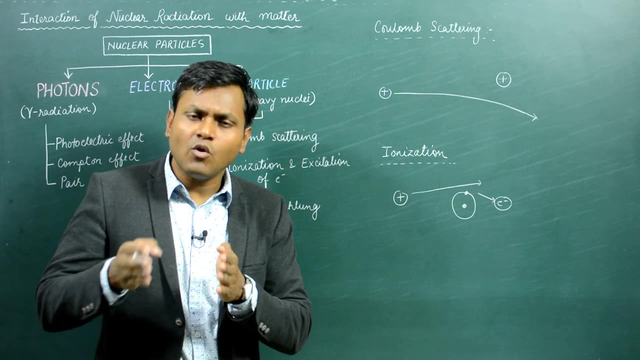 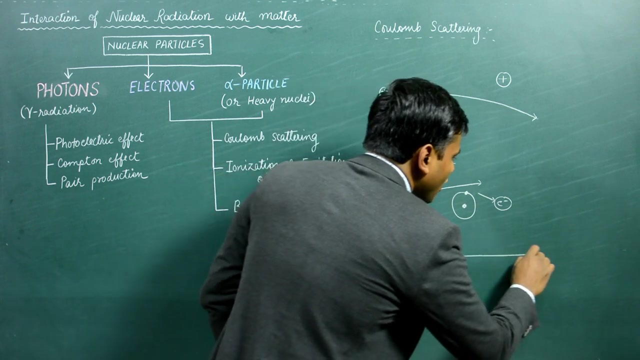 it usually leads to hundreds or even thousands of collisions along its path, where it transfers the energy to electrons and makes the electrons free in very small, small steps or very small, small decrements. So as the alpha particle is moving along a particular path, then it transfers its energy via. 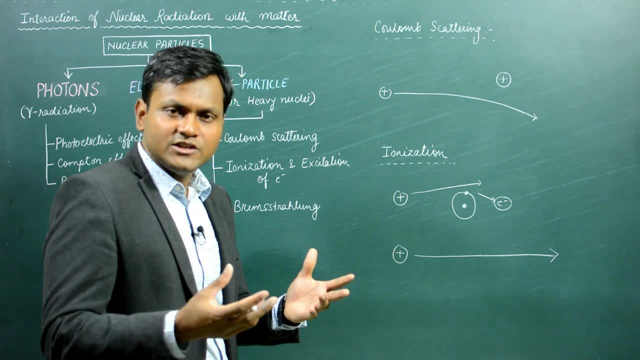 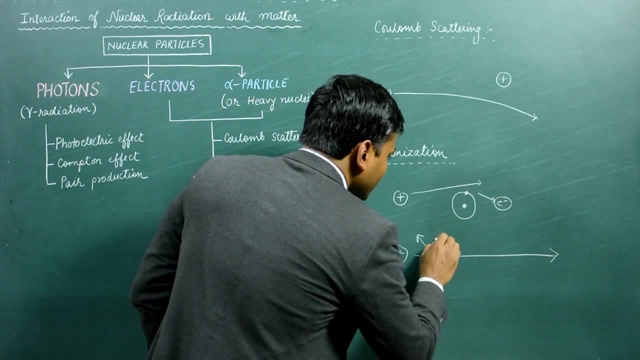 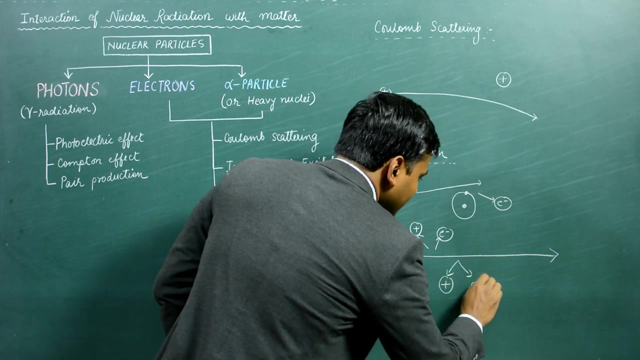 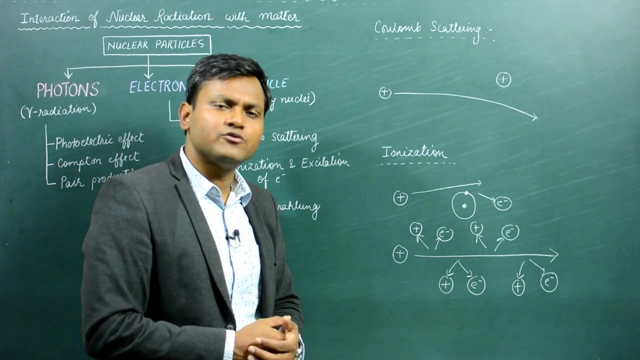 collision to the material medium and leads to the creation of free electrons and ionized or positively charged nuclei. and so in this process you end up getting the creation of target nuclei and free electrons along the path of the alpha particle. so an alpha particle might lead to the creation of hundreds of such pairs of free electrons and ionized ions. 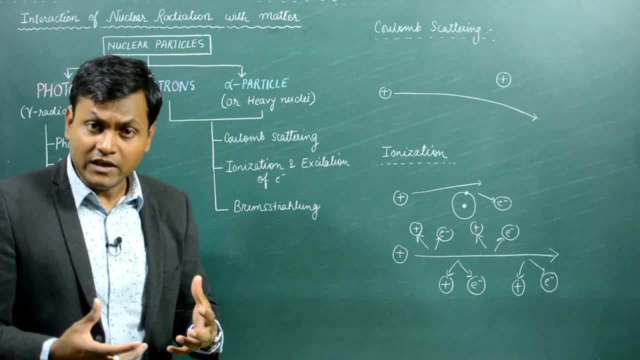 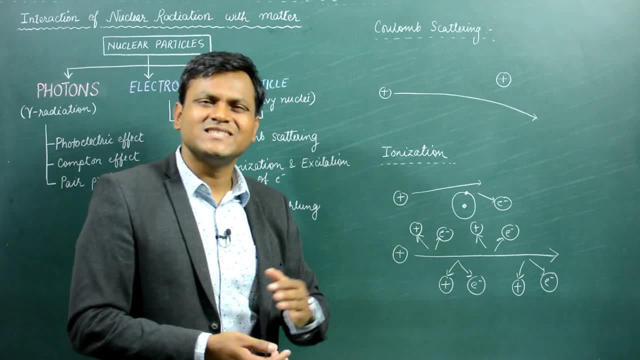 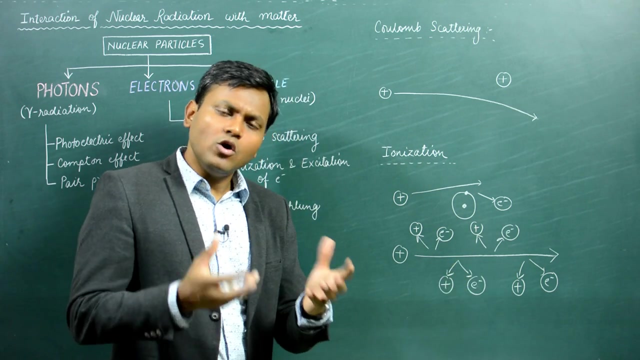 along its path because an alpha particle is heavy it and it has huge amount of kinetic energy. it usually does not get deflected along the process and usually moves along a straight line. it loses its energy slowly, slowly, in small decrements. with every single collision takes, that takes place the loss of 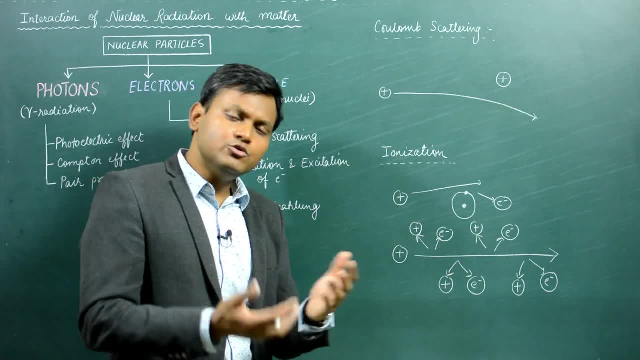 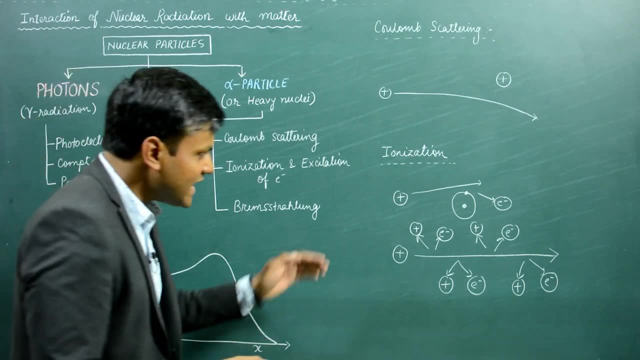 energy of an alpha particle as it enters a material medium is usually given by what is known as the Bragg's curve. so the Bragg's curve basically shows what is the amount of energy loss that happens as an alpha particle enters a material medium. as you can see from the graph here, the loss of energy is usually: 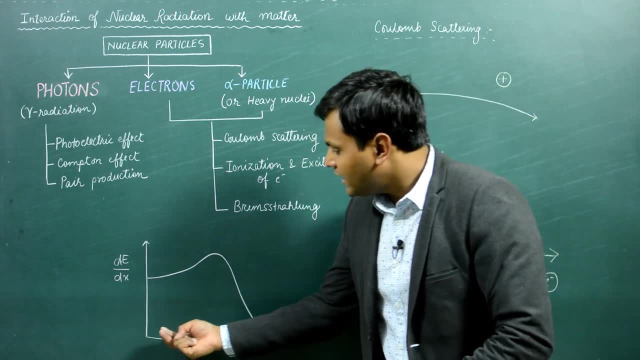 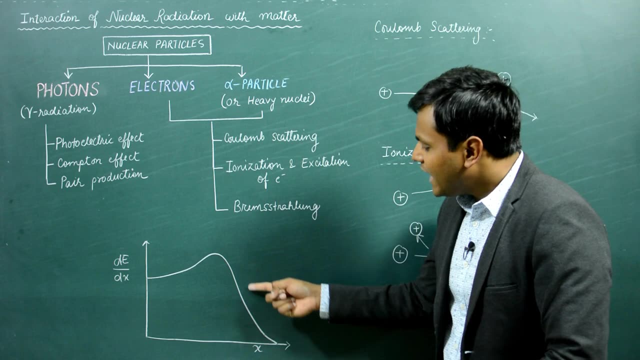 where, somewhere in the mid-range initially. and as the alpha particle enters inside the material medium, it will slowly lose its energy and the material medium that by the end of his journey, it starts losing more and more energy and it reaches a particular peak and it suddenly drops to zero. now why? 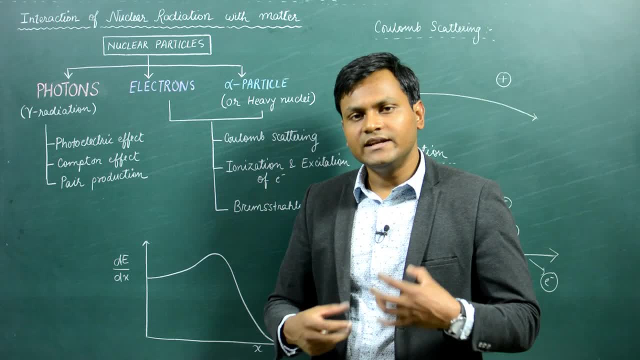 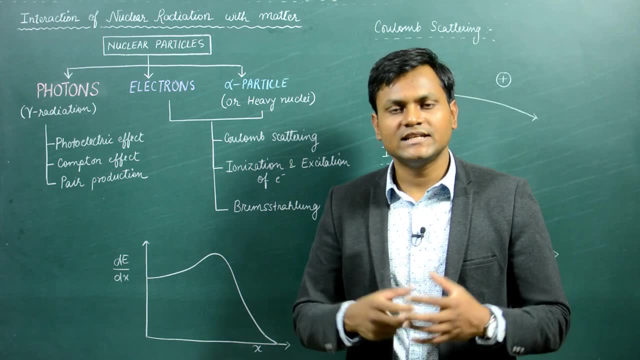 this happens it is because initially, when the alpha particle is entering the material medium, it has very high amount of kinetic energy, so it is moving at very fast velocity. since it's moving at very fast velocity, it does not get enough time to interact with the material medium and therefore the loss. 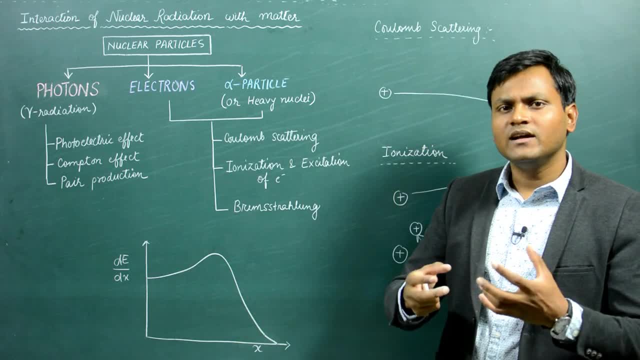 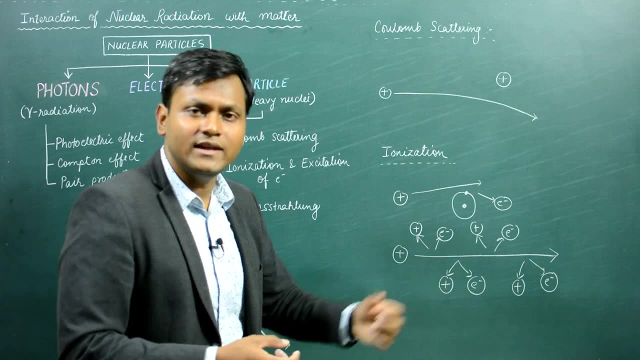 of energy is less as the alpha particle slowly interacts with the material medium and starts ionizing the material medium and starts losing the energy in small, small decrements than the velocity of the alpha particle decreases. The velocity of the alpha particle decreases. and now the alpha particle 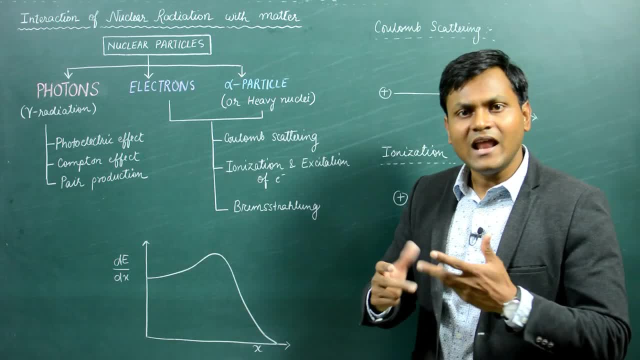 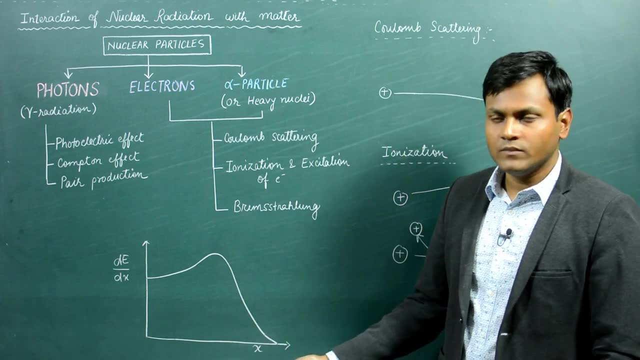 starts spending more time in the vicinity of the target nucleus and now suddenly, near the end of his journey, it loses vast amounts of energy and then suddenly comes to rest. so, as opposed to a photon, or even sometimes electrons, the alpha particle, which is a heavy particle and has a huge 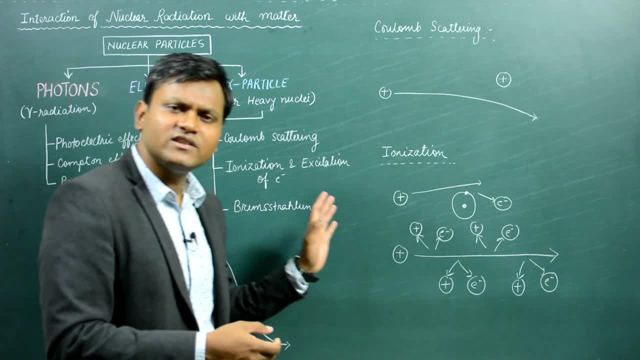 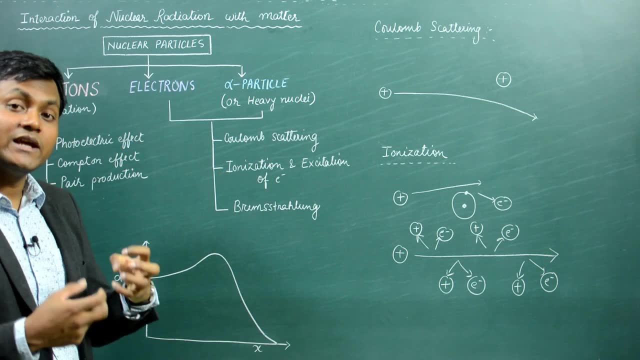 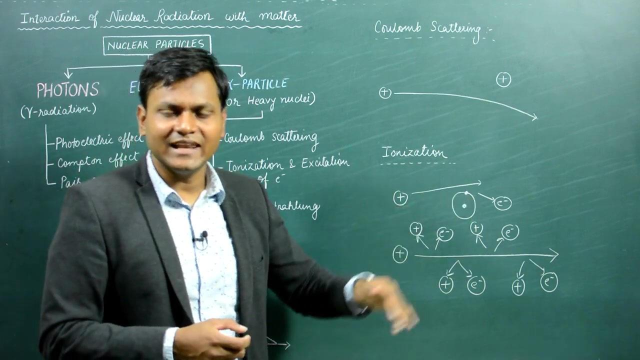 amounts of kinetic energy usually leads to creation of hundreds and even thousands of ionization along its path. This kind of anionization is also seen for extremely high energetic electrons, but electrons, being extremely minute and tiny particles, do not necessarily travel in a straight line, but they rather travel in zigzag lines. 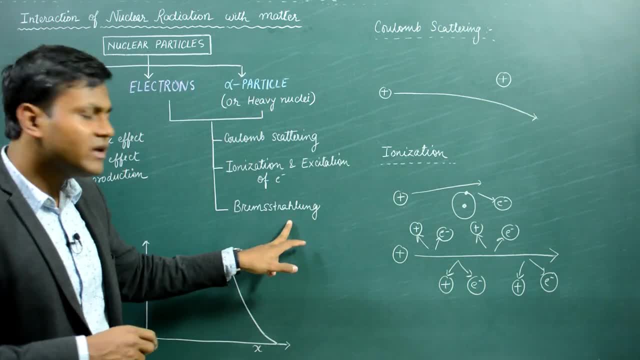 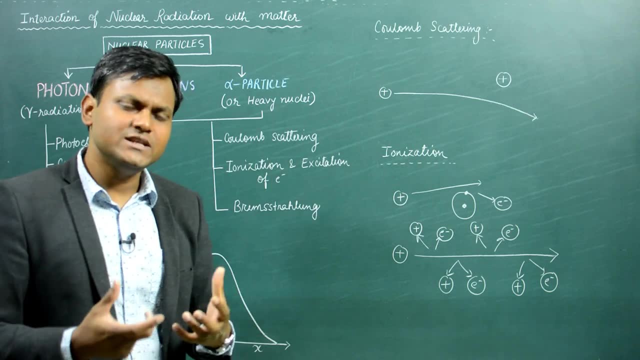 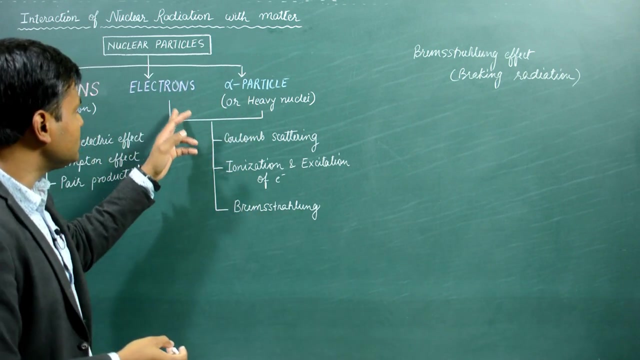 Finally, we come back to the phenomena of the Bremsstrahlung effect. So the Bremsstrahlung effect is exclusively shown only by electrons. This effect is shown whenever electrons come in the vicinity of some kind of a positively charged nucleus. So Bremsstrahlung effect of breaking radiation is usually seen whenever electrons are decelerated. 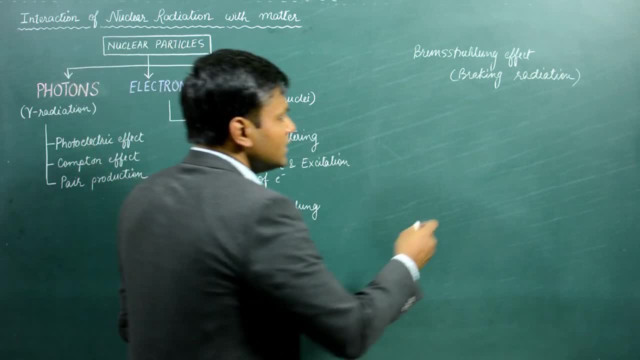 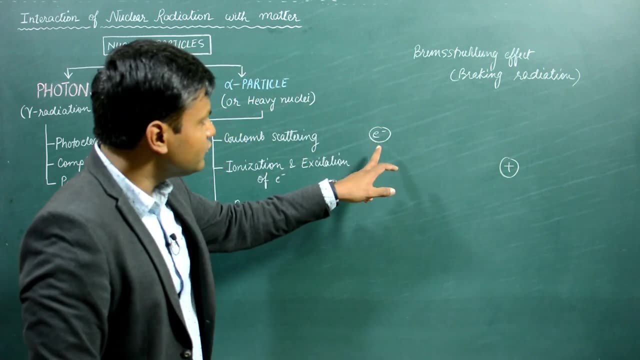 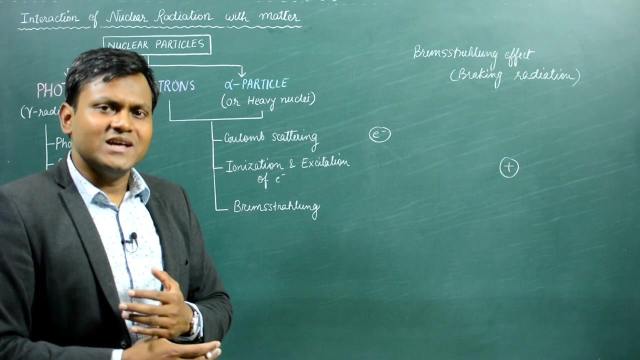 by some kind of a target positively charged nucleus. Now, you probably already know that when electrons come in the vicinity of some kind of a nucleus, since electrons are negatively charged and the nucleus is positively charged, the nucleus attracts the electron. What this attraction does is that it can change the trajectory of the electron. 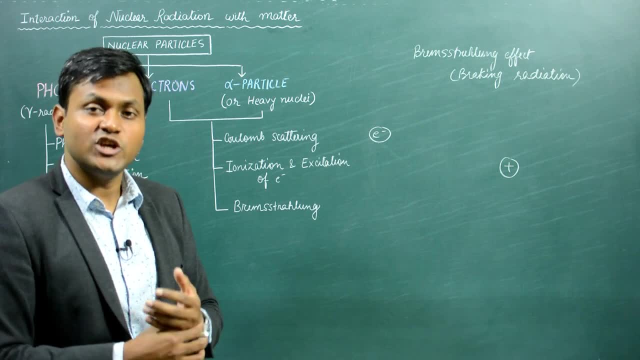 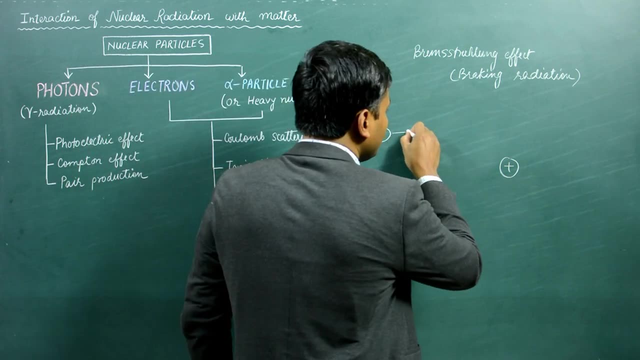 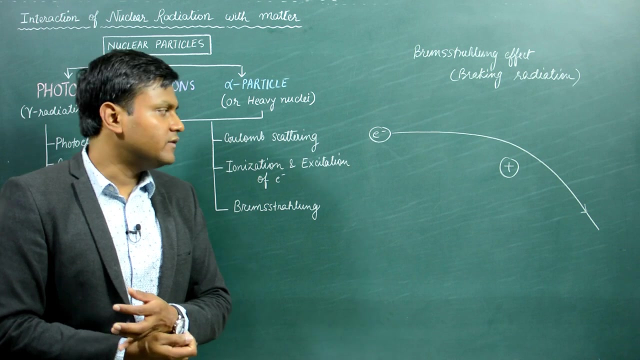 Now electrons being charged particles, and whenever charged particles get changed in its direction Or gets decelerated, it might lead to the emission of a photon. So if an electron comes in the vicinity of a nucleus then the direction of the electron might change due to attraction with the potential of the nuclear field. 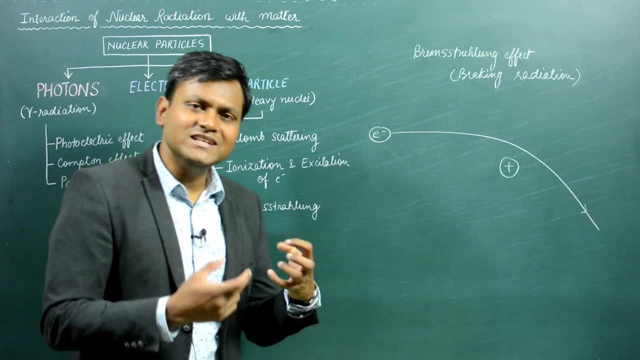 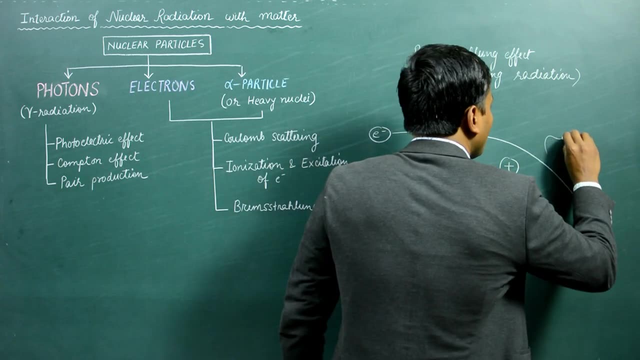 Now, because the direction of the electron changes. this might lead to deceleration of the electron, and deceleration of the charged particle always leads to the emission of some kind of a photon. So whatever photon is getting emitted will have energy which is basically equal to the